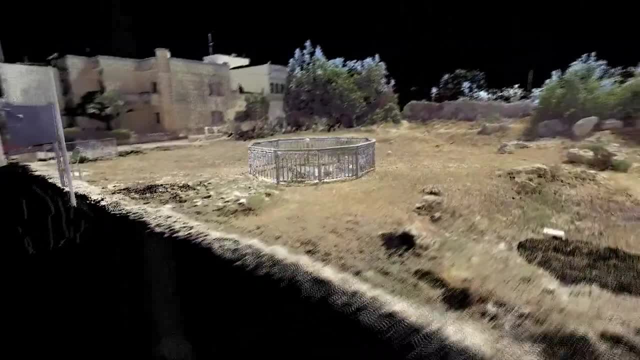 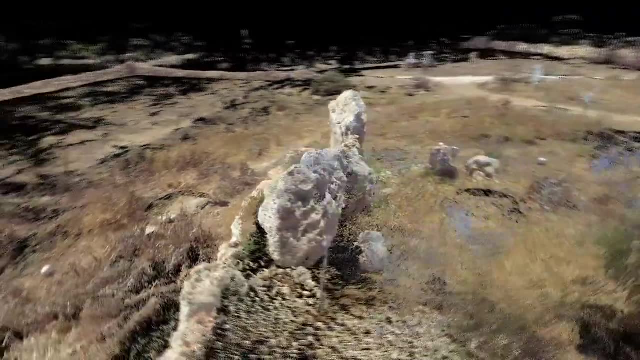 and that's the type of thing we're providing them with here in Queen's. It's about you, as a student, developing skills in those emerging areas, in those really exciting aspects of new archaeology that are really changing the way we think about the past. 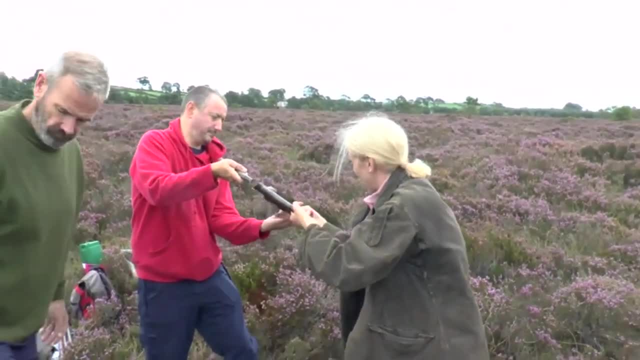 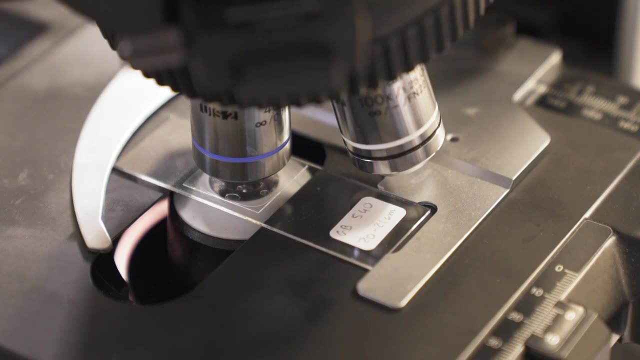 We're not just a school of archaeology, we're a school of archaeology and paleoecology. Paleoecology is the study of past environments, so we look at all aspects of environmental change and ecological change, climate change. So we're not just studying past peoples, we're studying how past peoples engaged within their 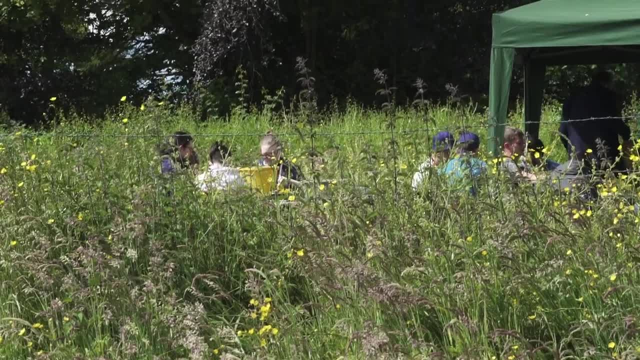 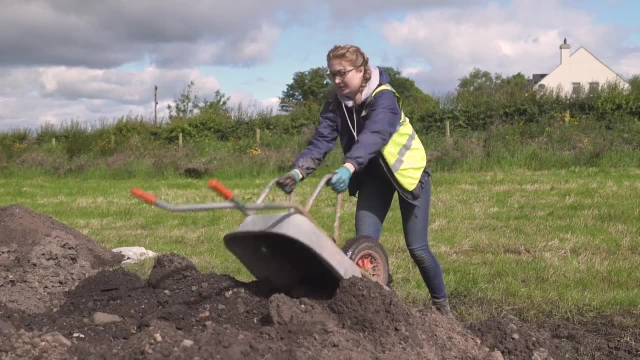 landscapes. We're only one of two or three departments throughout the UK that actually has its own dedicated field unit And they spend a lot of time in the field. They spend a lot of their time out digging things up. There's not many places that offer you the opportunity of practical experience, which 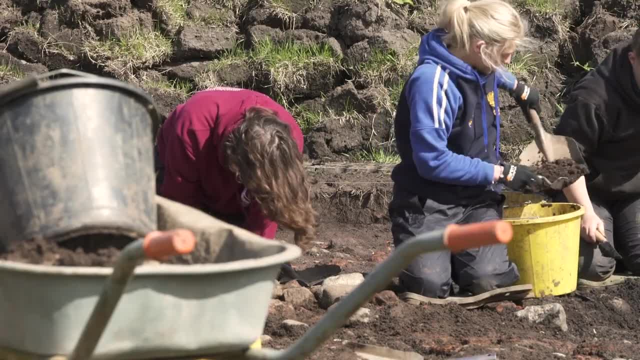 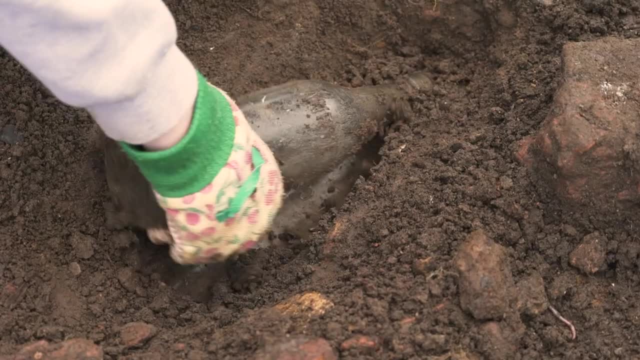 is second among. here at Queen's We learn how to dig and we learn the correct way to lay out the trench using GPS. It teaches you all of the basic skills you need to be able to go and work in archaeology, So it's a very practical hands-on course. 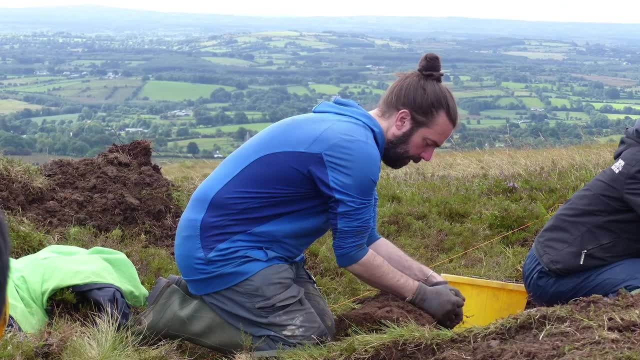 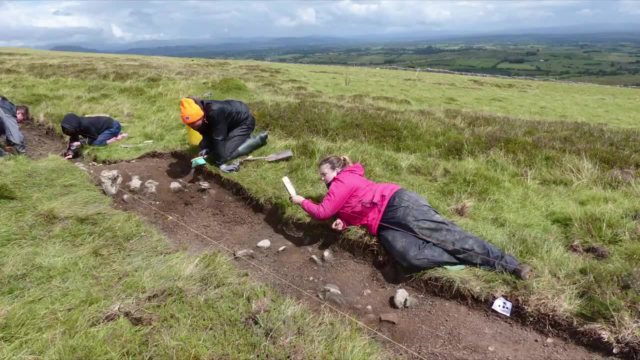 Lots of the fieldwork projects would focus on Second and Severick on the north coast, Navan Fort in County Armagh, the Rock of Cashel down in County Tipperary and L'Agour Cranach. They are four iconic sites. 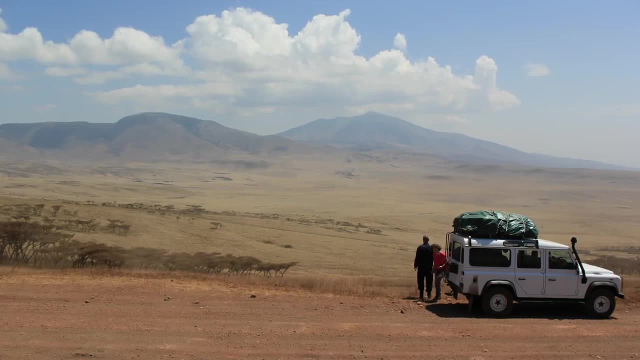 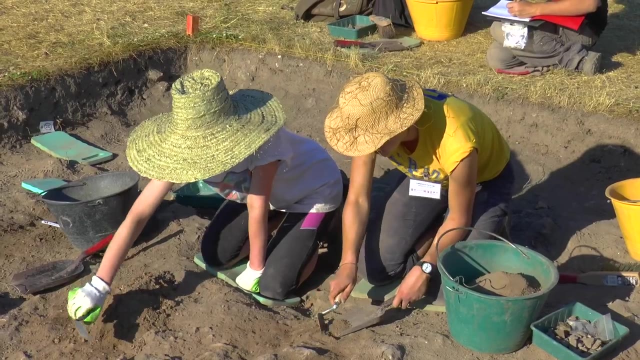 So to have a chance to go and explore, To go and excavate there is quite exciting. We also make sure our students have a lot of chances to travel abroad. If staff are excavating abroad, for example in places like Malta or Vietnam, there's always. 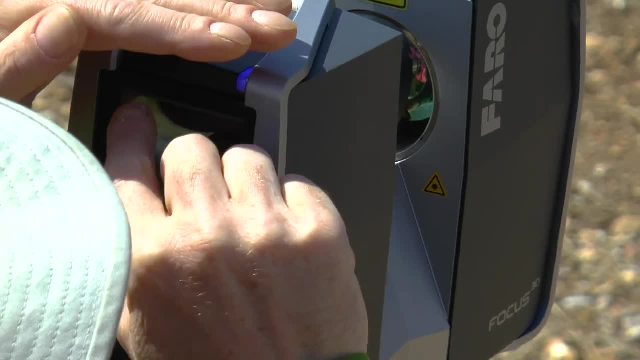 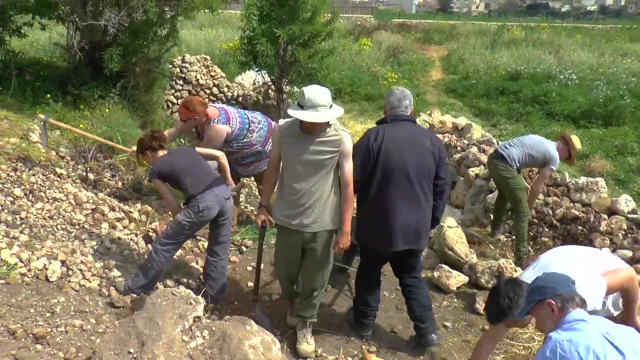 an opportunity for students to get involved too. I was able to go to the south of France and dig for a couple of weeks, which was really good. The other thing about a lot of these skills is that they're highly transferable. So, whereas the vast majority of our students do stay working in the heritage sector, a 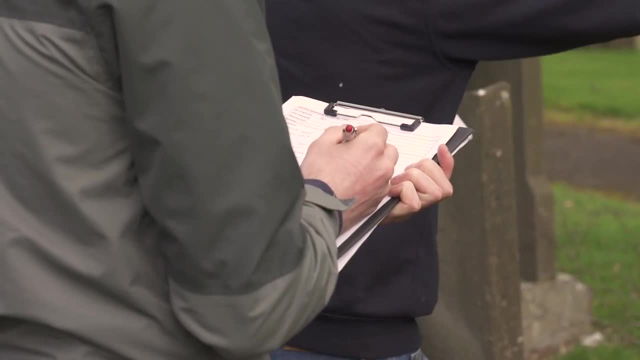 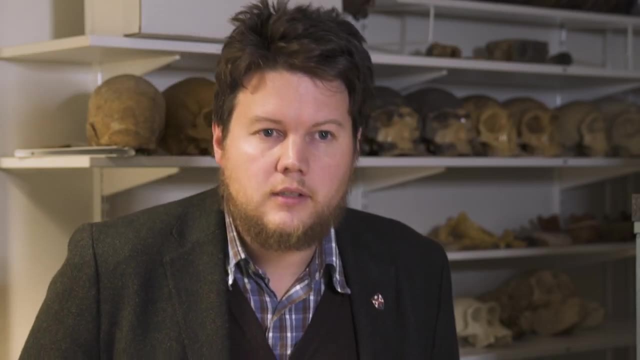 lot of them. take the skills they've learned, like mapping or survey, and they'll go and they'll get jobs in other disciplines which actually use those skills. Culture is what makes humanity different. The things of the past form who we are, and if we lose sight of that, we really lose sight. 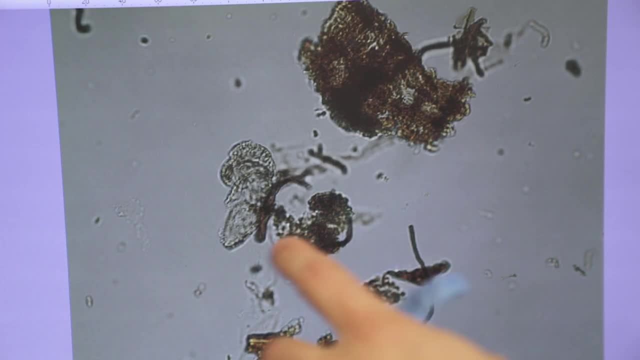 of who we are as people. Archaeology holds up a mirror to contemporary society, and it allows us to reflect on our place in the world as we are now and where we want to go into the future.